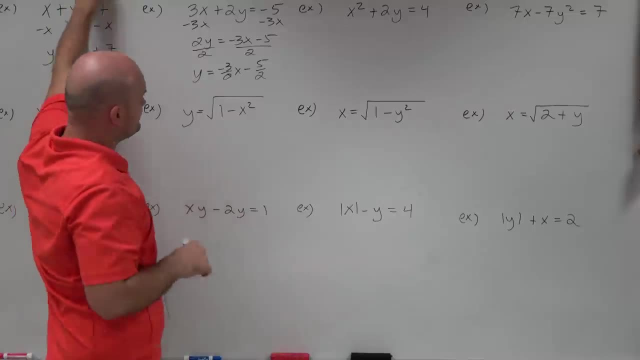 halves x minus five halves. Um, But again, by science solving, I solve for y and it's still producing y uniquely. So therefore, again, this is just a function. Now, in this next example, you see an x squared. 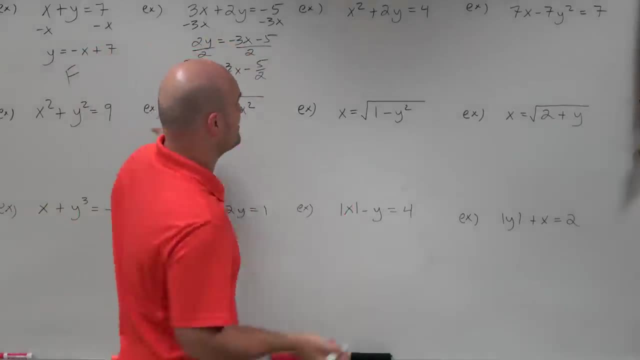 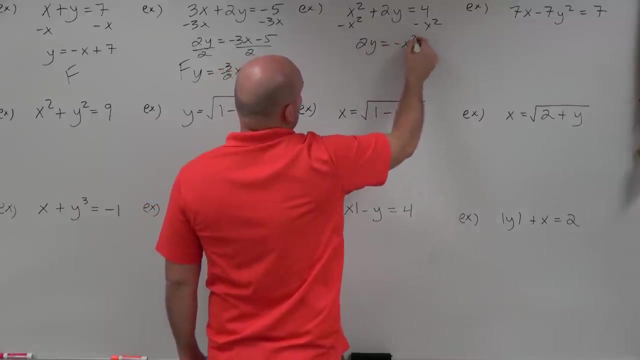 So this is going to start coming into some issues for us. But in this exact problem again to solve for y, I don't really need to do anything crazy Again. I can just use my inverse operations and everything really kind of works smoothly here. 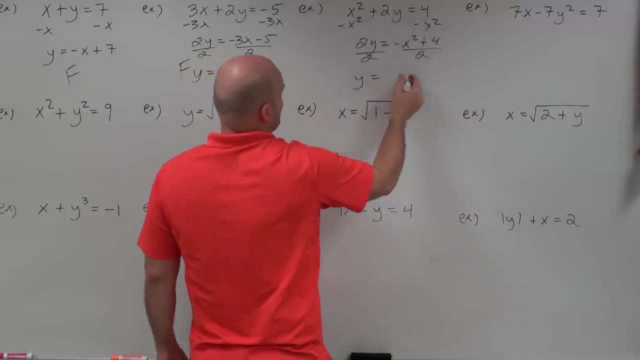 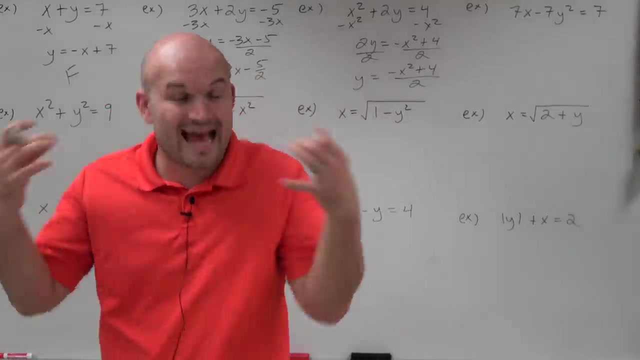 Divide by 2, divide by 2.. Here I separated them. For this one I'll just leave them together. But again, every single time I plug in a number, in for x, any number I plug in, And if you're having trouble wrapping your head around this, 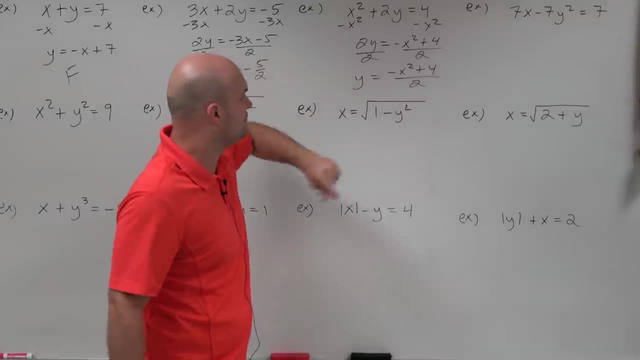 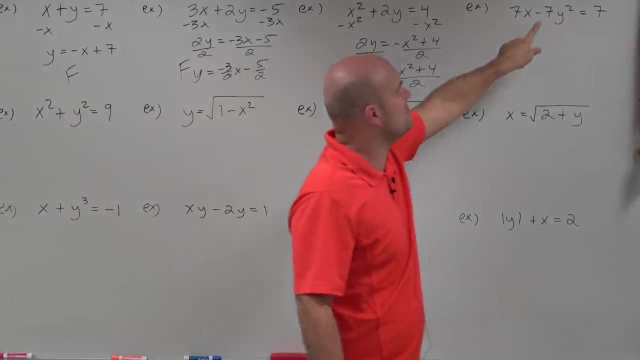 just pick some random numbers, Plug them in for x. Every single time you plug them in for x, you're going to get one unique y Over here. same thing, but now you can see that my y is squared. So when I'm following my inverse operations, 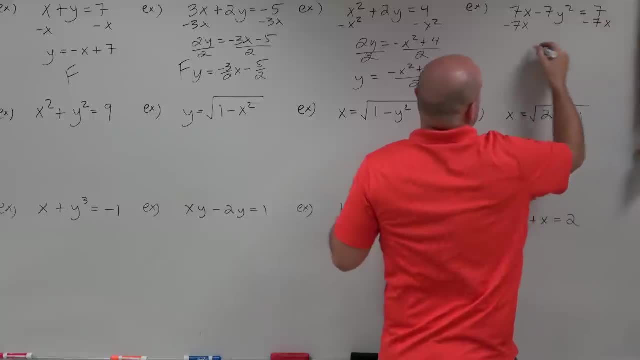 I'm going to do the same thing. I want to isolate the y. But when I isolate the y, I'm going to make sure that I'm solving for y uniquely. So I divide by negative 7,. divide by negative 7.. 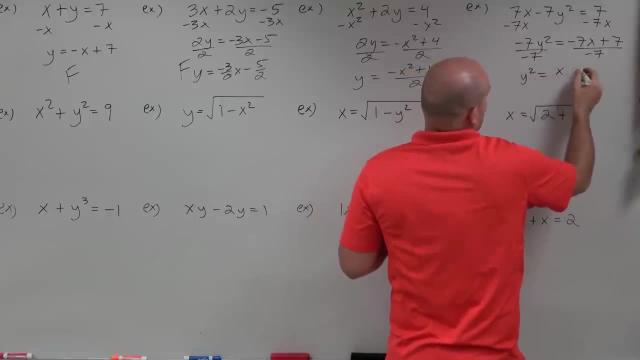 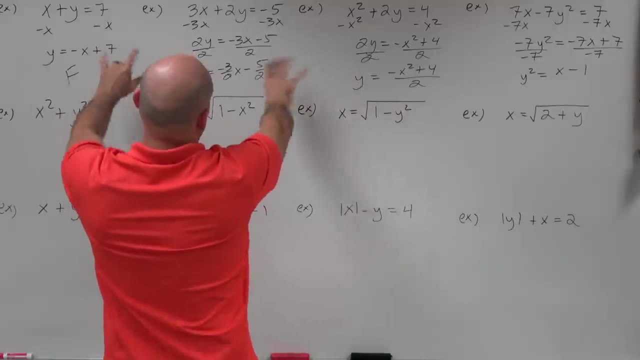 And then I have y squared equals. let's see that becomes an x minus 1.. So now I've applied all my inverse operations, But the only inverse operation I have not gone into so far I've just been add, subtract and multiplying. 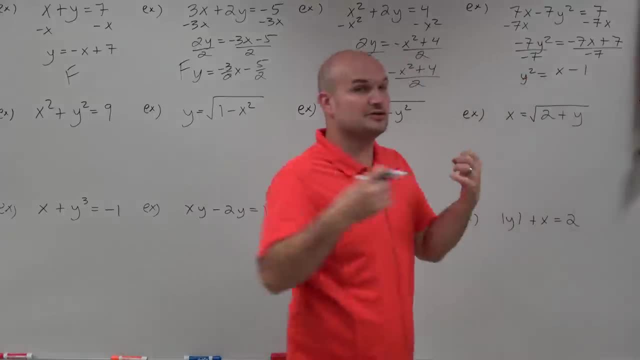 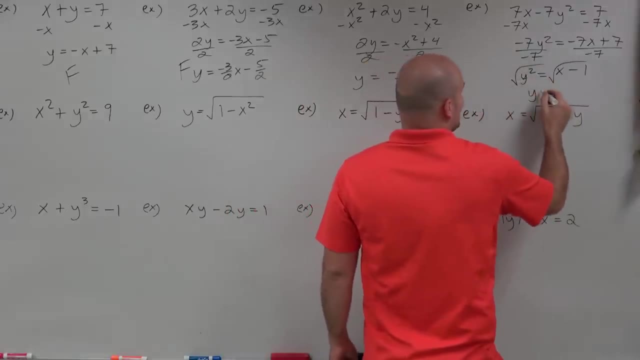 But now you can see my inverse operation here is squaring. So to introduce to undo squaring I need to take the square root, But the inverse operation here is squaring. So the issue here now is when I introduce the square root. 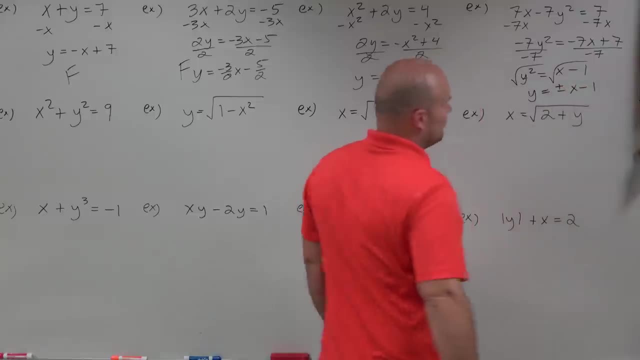 I now have to include plus or minus x minus 1.. Sorry, that's still the square root of x minus 1.. And the purpose of that goes into just kind of go back to: let's solve for x squared equals 4.. 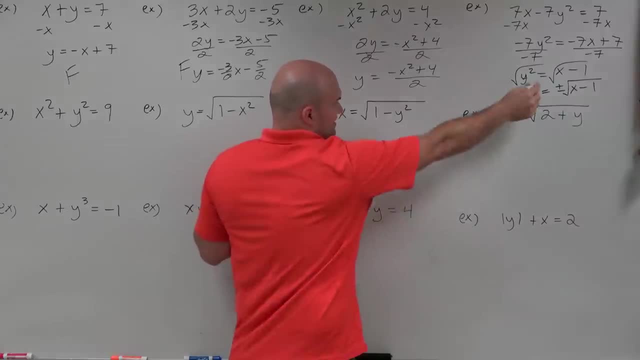 Well, this has two solutions. Now I'm solving for x. Well, let's just pretend This one might be a little more difficult. So let's look at y: squared equals 4.. If I wanted to solve for y, here you'll. 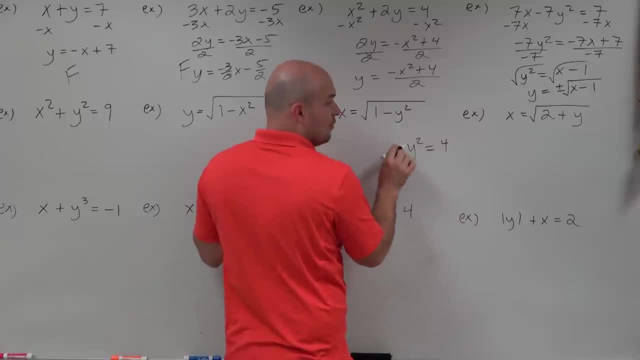 notice that this is not two unique solutions. There's not one unique solution for y, Because when I subtract this, I have y equals plus or minus 2.. And the reason being is because if you were to plug in positive 2 and for y, you'd get 4.. 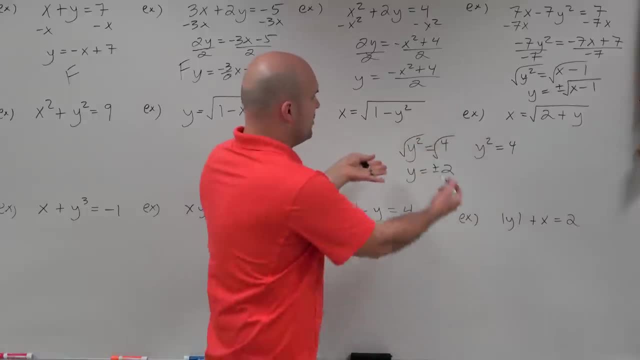 If you were to plug in negative 2 and for y, you would still get 4.. So when you introduce the square root, you have to include plus or minus. But what the issue is, what that means, is this: y is now not unique. 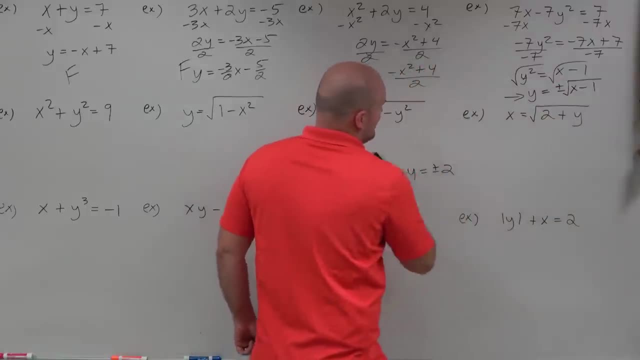 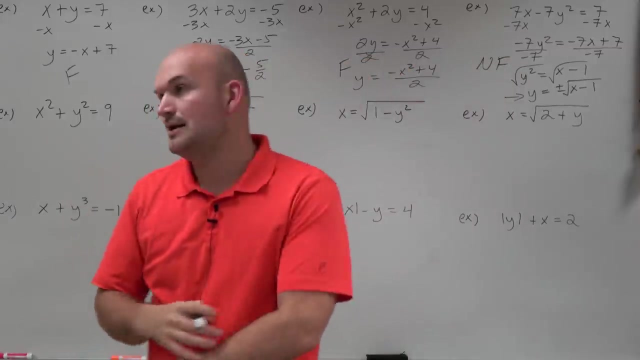 There are now two different answers for this case. So therefore, since my y is not unique, this is not a function. OK, Then we get into one over here where x squared plus y squared equals 9.. Hopefully, maybe in geometry class you remember what this function looks like. 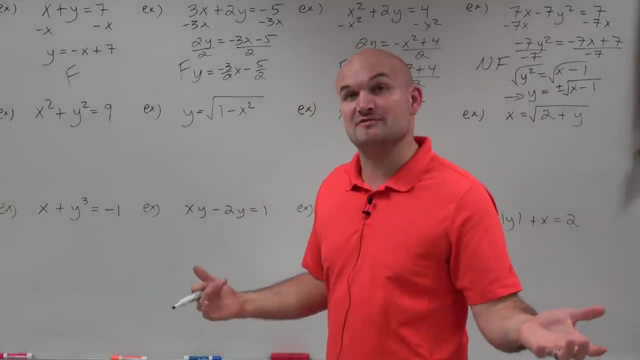 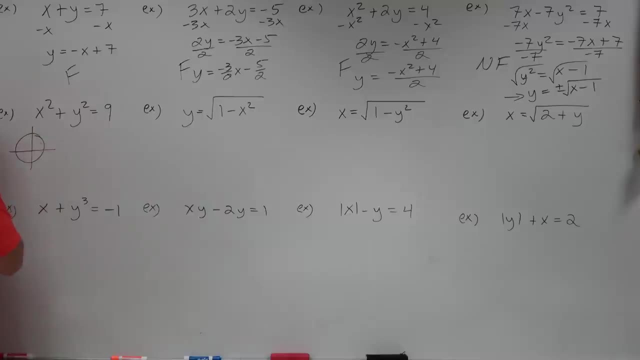 This would actually provide a function of a circle. So if you actually know with a radius of 3, you would actually already know that this does not pass the vertical line test. However, if we just wanted to look at this, let's again do the same thing. 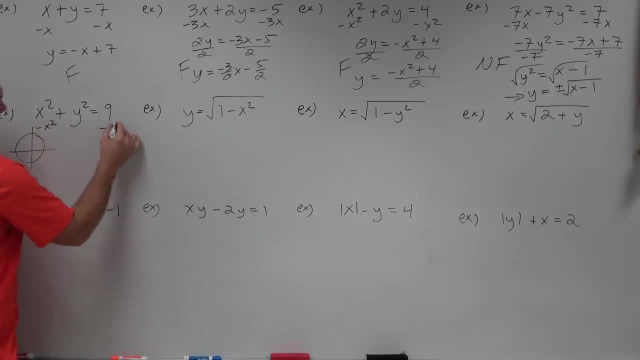 Subtract the x squared on both sides And we'd have y squared equals. let's do 9 minus x squared, plus y squared equals 9.. OK, All right. All right, 9 minus x squared. And again I have to undo the squaring. 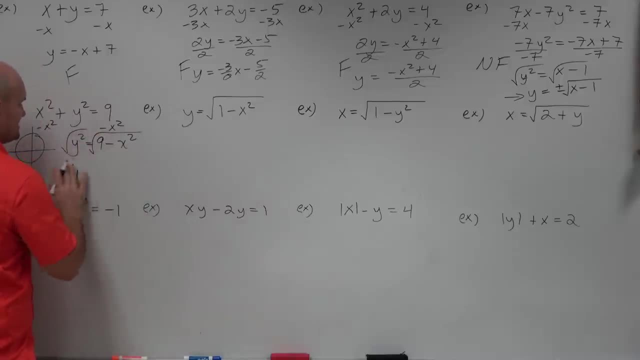 So when I undo the squaring I have to do plus or minus. y equals plus or minus the square root of 9 minus x squared. So again, since I do not have a unique y because there's two solutions, that is not a function. 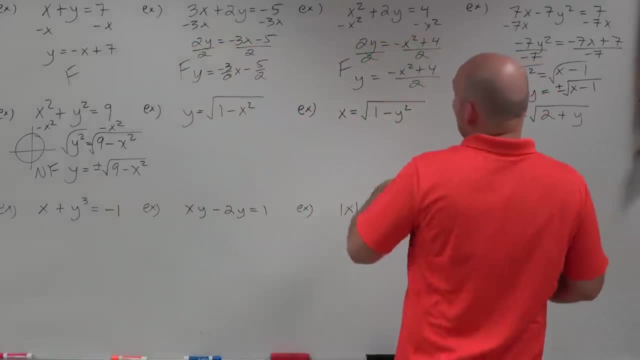 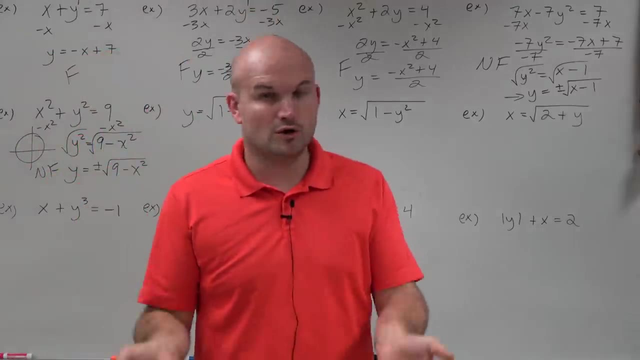 So the correlation that I want you to see is: as long as y is linear right now, so far what we've determined. as long as y is linear, we're good. It's a function, Doesn't matter really what x is. 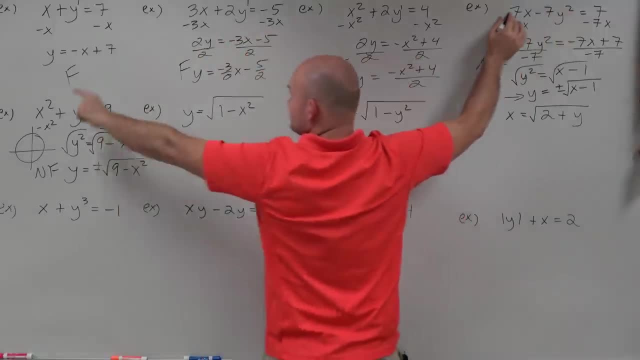 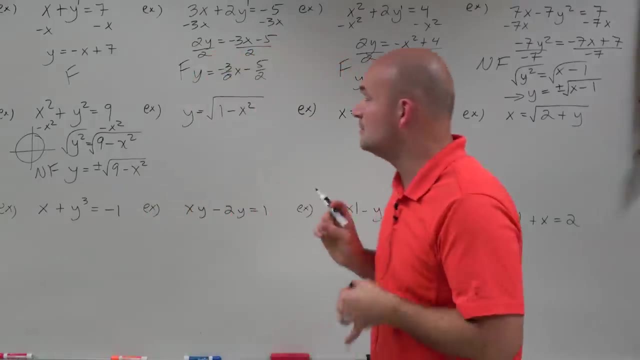 But as long as y is linear, it's good. When y is quadratic, or hence raised up to an even power, it's not going to be well. at least if it's from quadratic, it's not going to be a function. 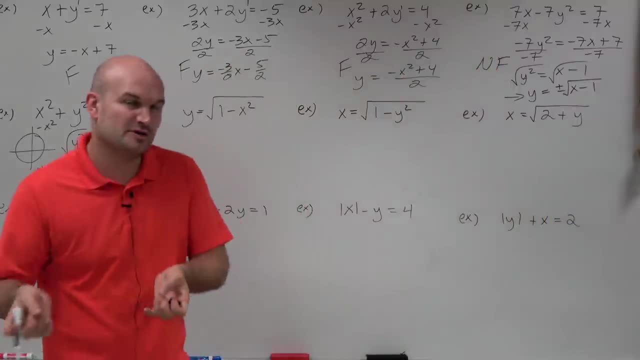 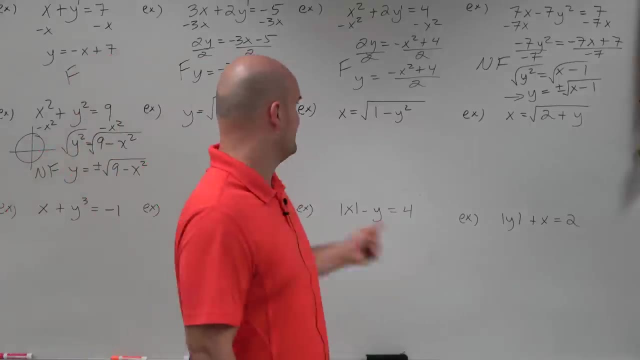 OK, Because therefore taking the square root, as I mentioned over here, is going to produce two different results. So therefore our y is not unique. Over here we see we have another square root. Kind of a little interesting. This is actually a very common function, that, or sorry. 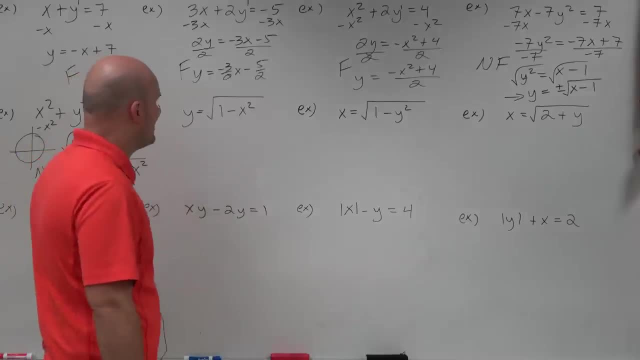 didn't want to give it away, But this is a very common equation that we will see quite a bit, But without graphing. if you don't know what the graph looks like, let's just use. what am I doing? Why am I always solve for this? 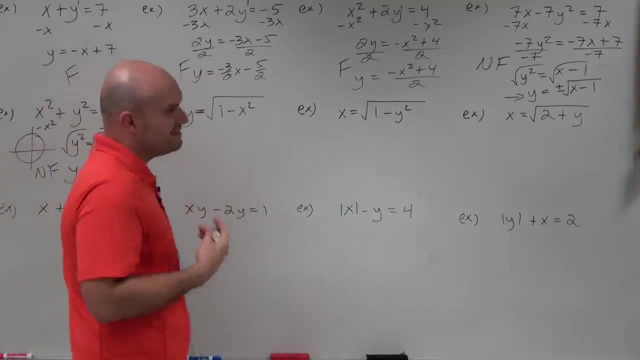 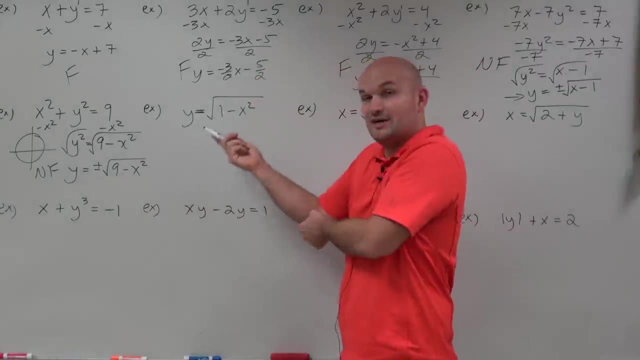 Oh, OK, All right. Well, yeah, I guess that was the problem here. So in this example I was getting ahead of myself. The reason why this is a function and this is not a function is because here we're just saying: just take the positive square root. 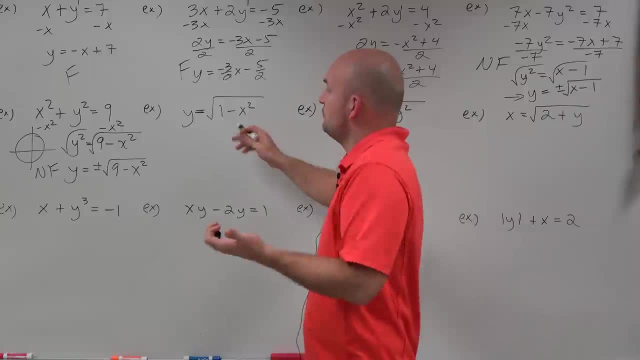 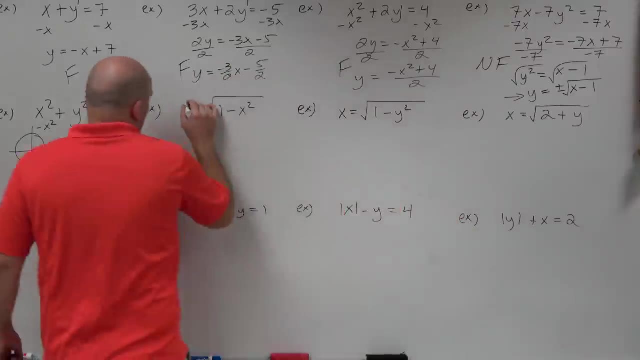 We're not saying plus or minus, We're just saying The square root, Positive square root of this. Or we could even say: take the negative square root, But it doesn't really matter. Either way, we know that y is already provided uniquely. 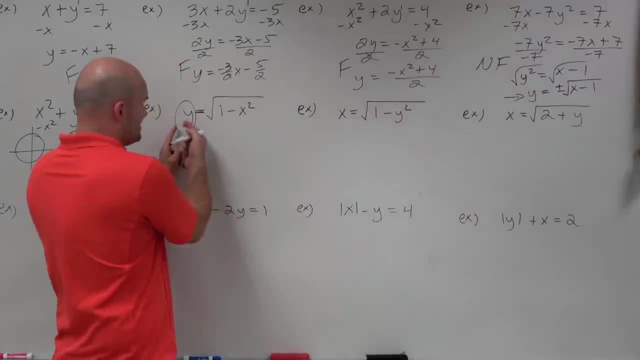 So, no matter what the equation is, as long as you have y already isolated and there's no y's over here at least- therefore, then you can just say that that is a function. It is already solved for y uniquely. So we're good to go. 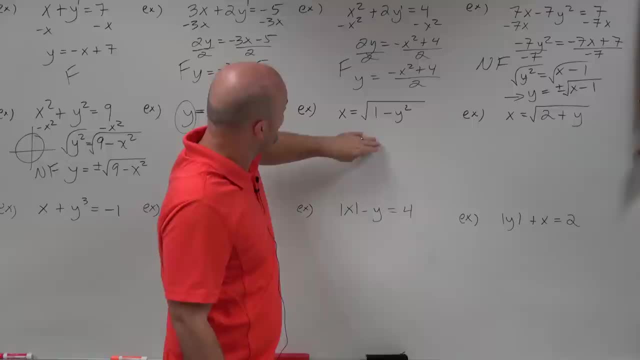 Here. these are the two examples. for some reason I was getting ahead of myself on These two equations we have to solve for our y Right. So to do that, what I'm going to do is I'm going to square both sides. 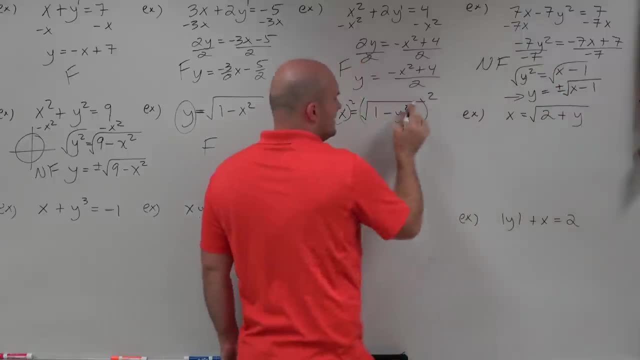 That's going to undo the square root. Just like how I had to undo square and I took the square root, here I have to undo square root, so I square both sides. Therefore, I'm left with x squared equals 1, minus y squared. 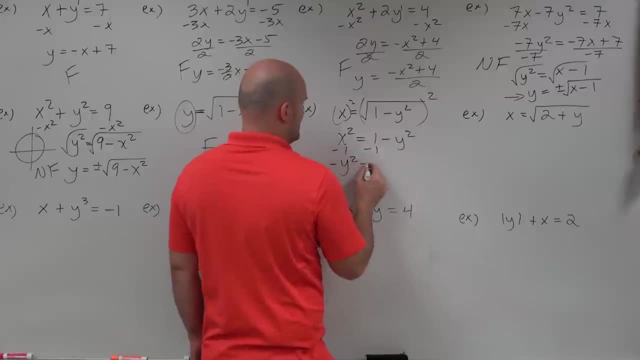 Subtract 1, subtract 1.. Let's replace this over here. Negative y squared equals x squared minus 1.. Divide by negative 1, divide by negative 1.. y squared equals x squared minus 1 over negative 1.. But again, you can see that since we're solving for y squared, 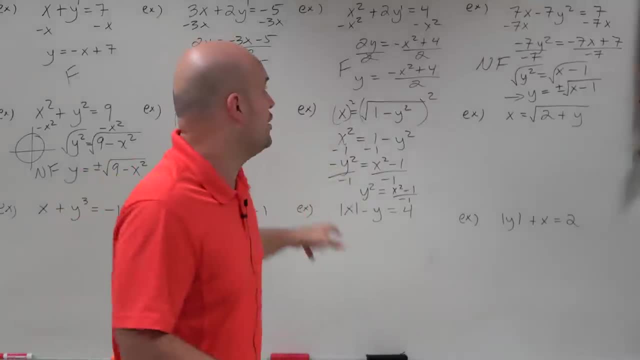 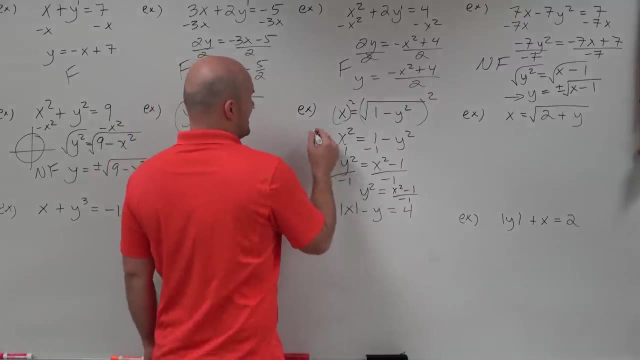 I've isolated my y and it's a y squared. I know from my previous results that whenever I'm solving for y squared, this is not going to produce a unique result. So this is again another example of not a function. 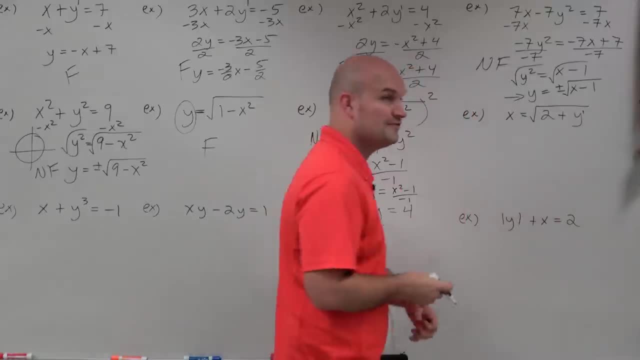 And last but not least, let's go ahead and do here. Now. we can notice that my y is to the first power, So I'm assuming it's probably going to be a function. But let's just solve it here real quick. 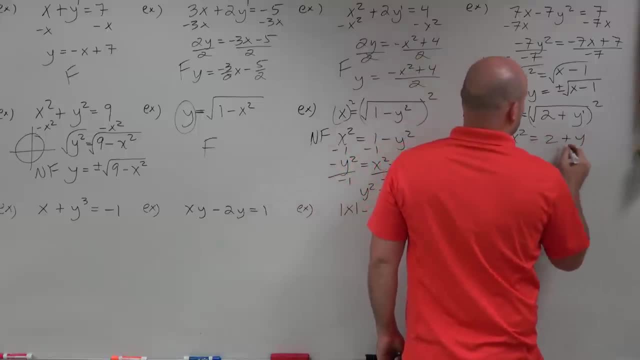 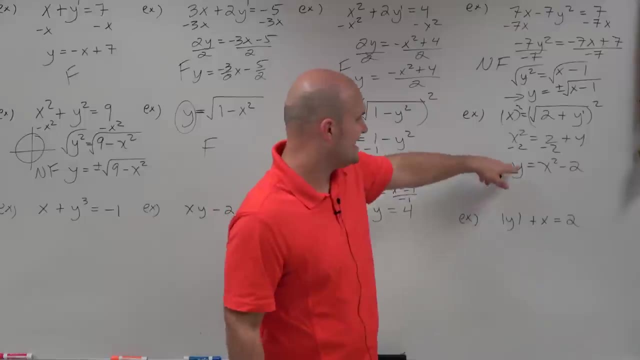 Square both sides: x squared equals 2 plus y minus 2 minus 2.. y equals x squared- x squared minus 2.. So, even though it was under square root, when I solve for the y, you can see I solve for it uniquely. 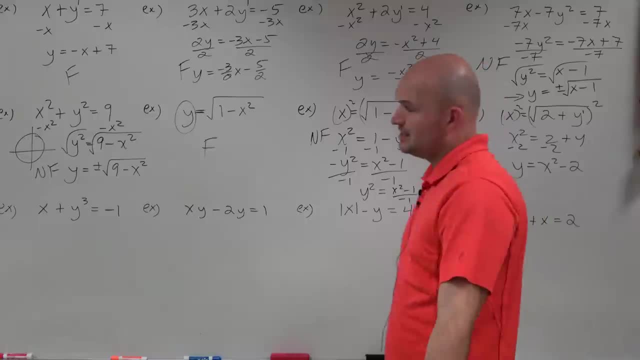 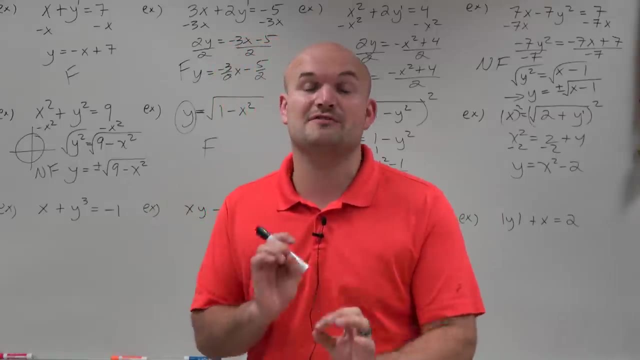 So it's all good. Now we said that quadratics do not when y is squared, then it's not going to produce a function, Because you're going to have to take the square root and you have to include even and positive and negative. 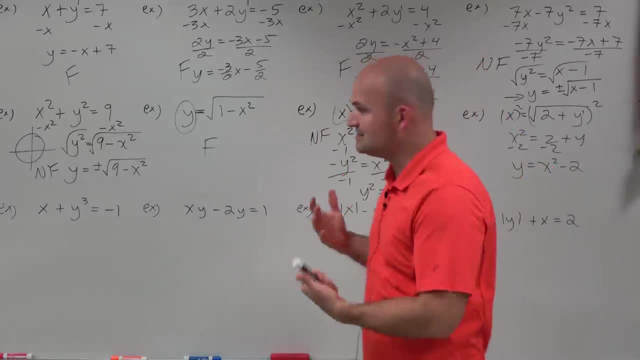 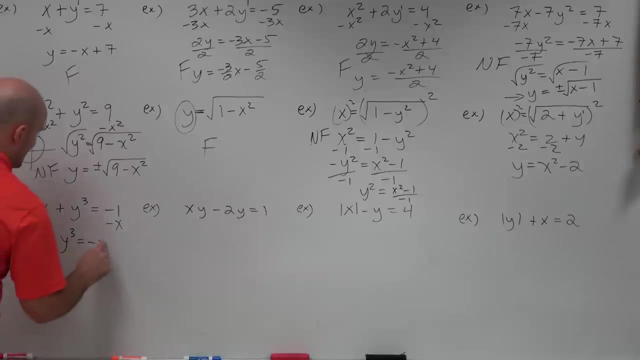 However, what about if y is raised to the third power? How is that now going to affect everything? Well, we're going to go ahead and subtract And therefore we have y cubed equals negative x, Negative x minus 1.. 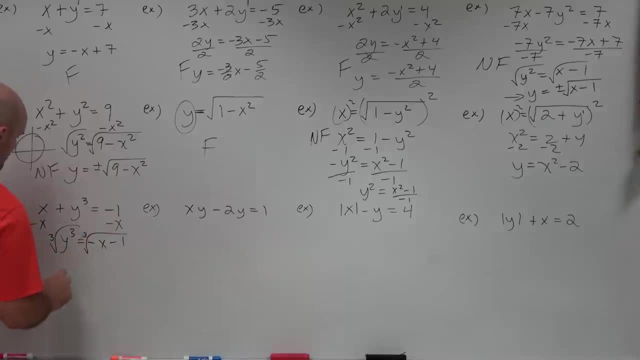 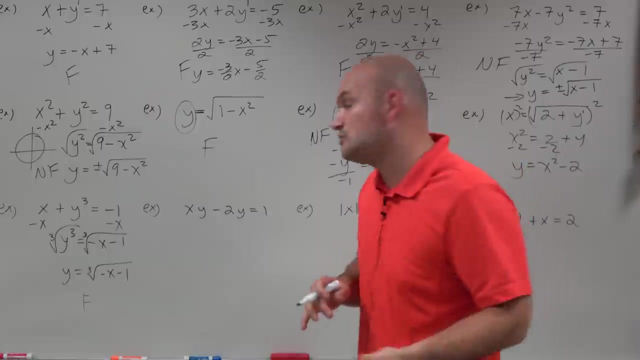 Now, when we take the cube root to undo cubing, we'll have y equals the cube root of negative x minus 1.. Now the important thing about this is this actually is a function, And the reason why comes into the understanding of cube roots, how they compare from square roots. 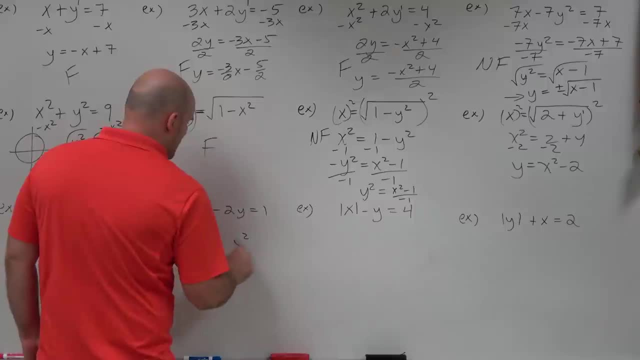 So let's look at again x squared. I'm sorry, let's do y. y squared equals 8.. I'm sorry, not y, 4. So when I go ahead and solve this, y equals Plus or minus 2.. 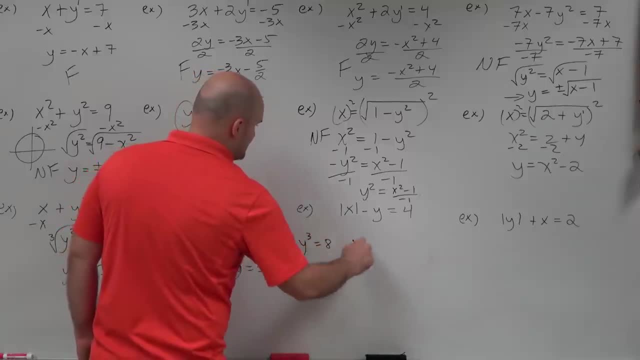 Well then, let's look at: y cubed equals 8. And y cubed equals negative 8. When I take the cube root here- so I take the cube root of both sides- I get y is equal to positive 2.. 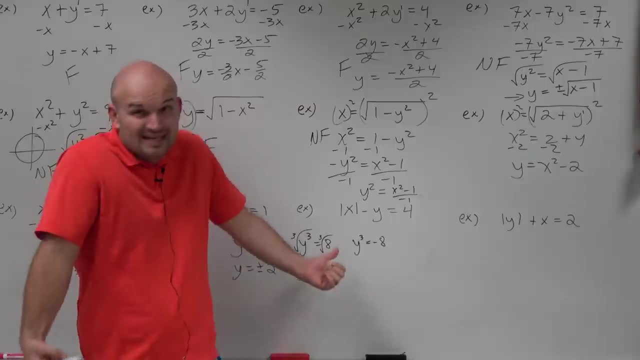 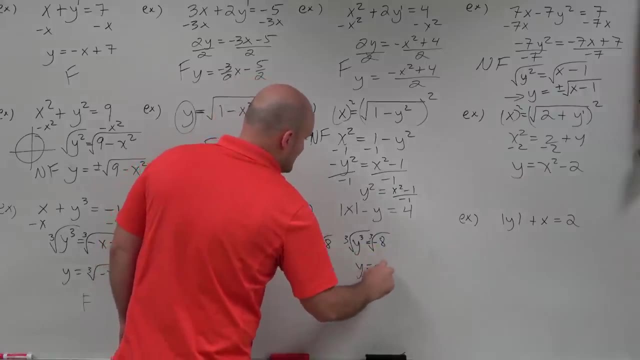 Because the only number that multiplies by itself three times to give me positive 8 is positive 2.. In the same respect, when I take the cube root of negative 8, I get y equals negative 2.. Because negative 2 is the only number that I multiply. 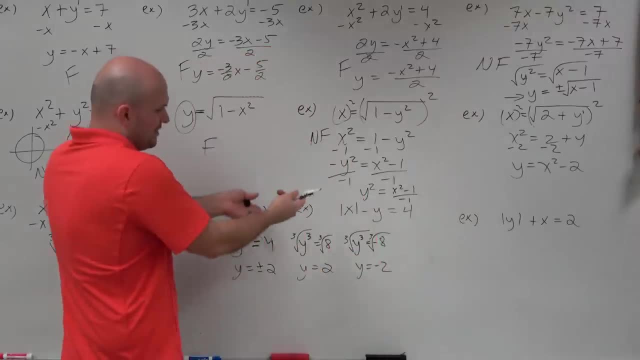 by itself three times to give me negative 8.. So what happens is when it's odd, I'm solving for y uniquely, But when it was squared, solving for y is not unique. So therefore, y the summary that we need to understand. 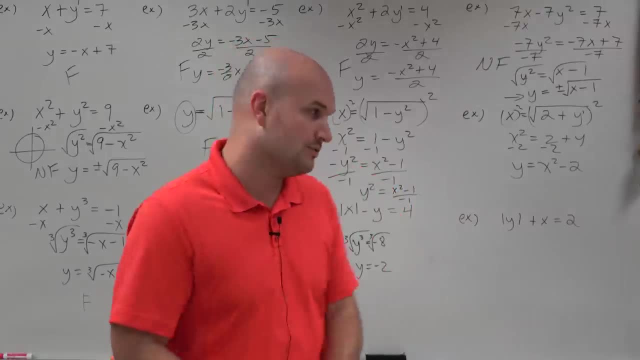 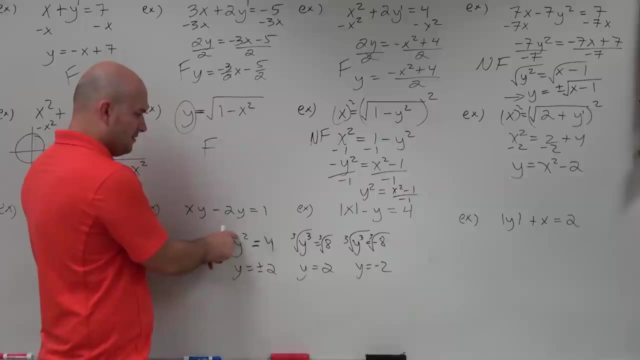 is y raised to any odd power is going to be unique when solving for it. So therefore it is going to produce a function. However, when you have a y raised to a even power, it's not going to produce a function when you go ahead. 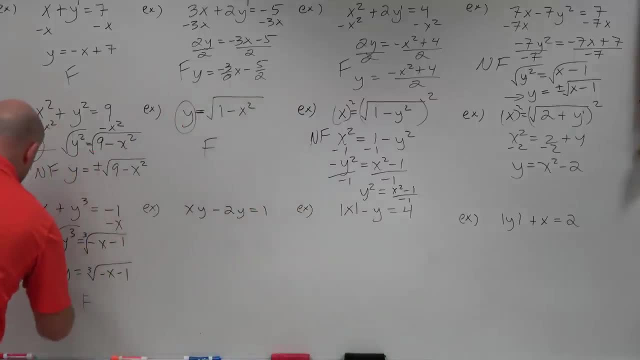 and solve for it. All right. So therefore, we can say that this is a function. Now let's move to the next one. Now we have two y's, And usually, when we'd want to solve for y's, this kind of produces a problem because, well, 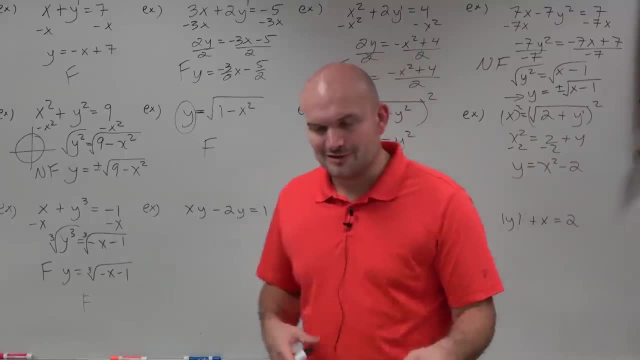 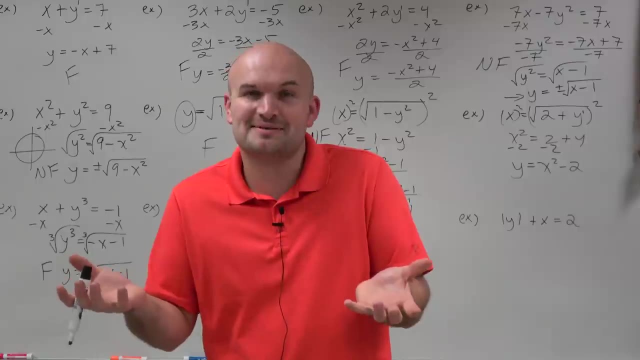 if we look at this, we can't combine these two y's. However, there's two ways to combine like terms. It's either combine like terms, combine them with like terms- I guess I have done saying that three times- or factor out a common term. 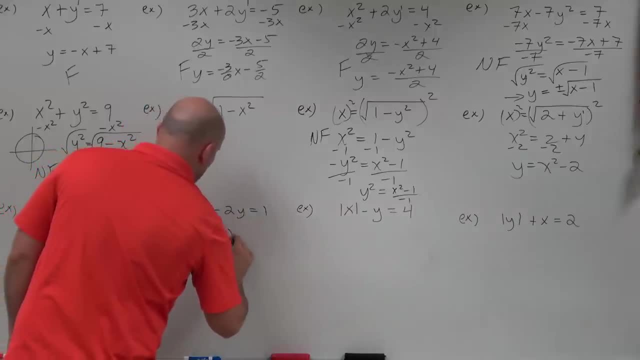 So if I factor out a- y, I get x minus 2 equals 1.. All right, Now I can divide by 2, or x minus 2. And I get y equals 1 over x minus 2. And that is solved uniquely. 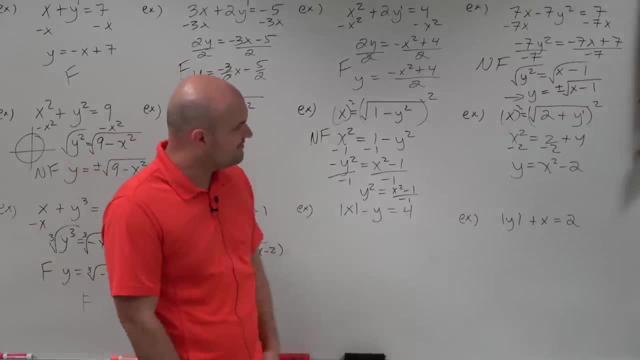 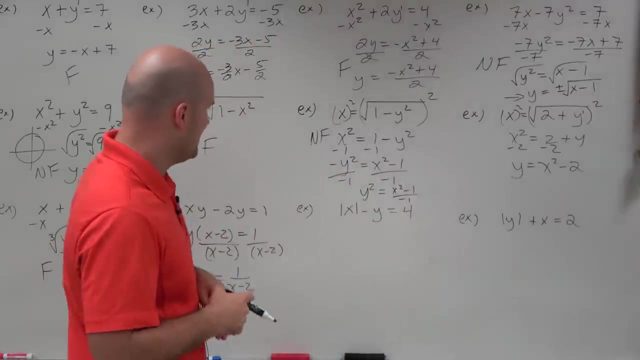 So we're all good, And the next one. now we're going to investigate absolute value. And again remember, absolute value is like the absolute distance away from 0. So I'll get into that a little bit more explanation here. for on the second problem, 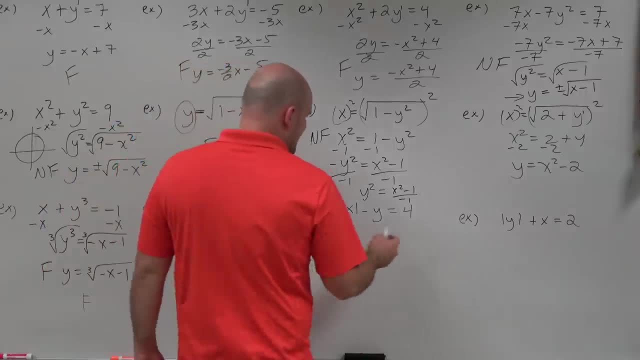 But for the first problem, I think we're going to solve this using our inverse operations, And actually what I'm going to do here is I'm just going to get the y to the other side, so I don't have to deal with negatives. 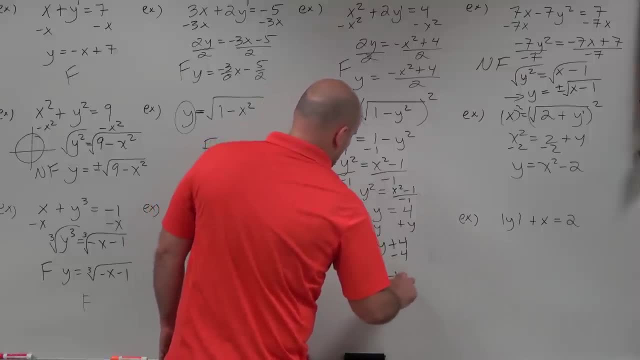 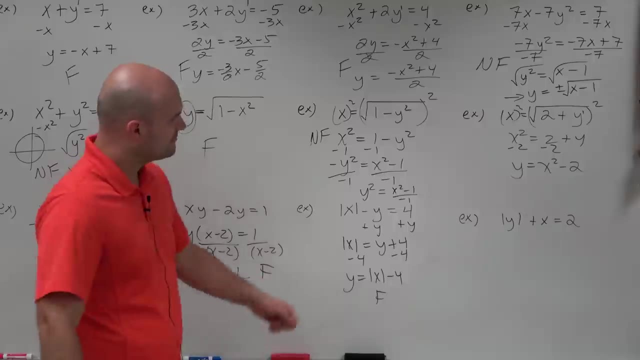 And just by using my inverse operations you can see that I can easily solve for y uniquely. So that is now a function. And that was a function too. I just forgot to write it. But now, on the last one, let's go ahead and look at here: 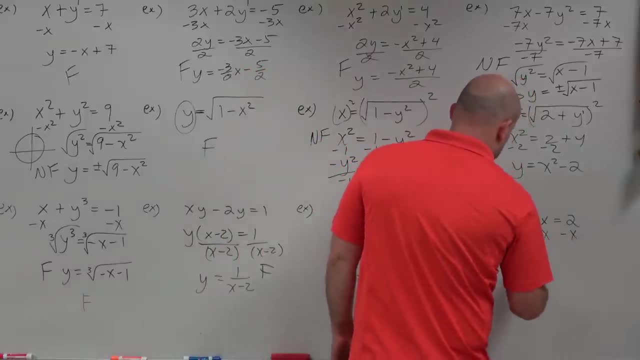 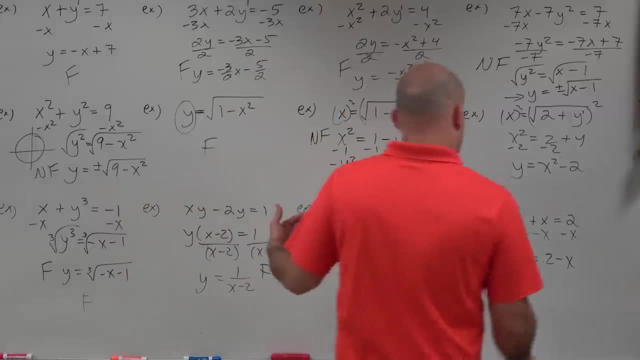 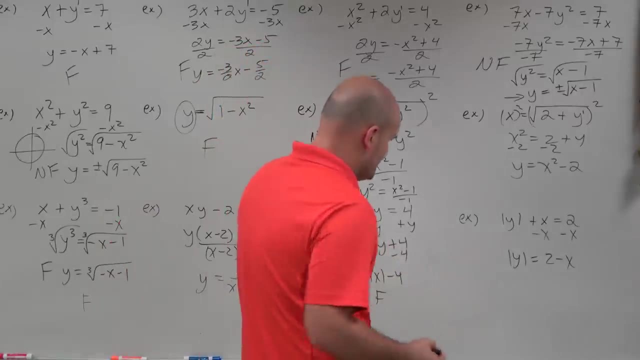 So the best way to do this is to do this. So the best way to do this is to do this. So the best way to look at this, if you remember solving for absolute value equations, let's look at solving absolute value equations, like absolute of y equals 4.. 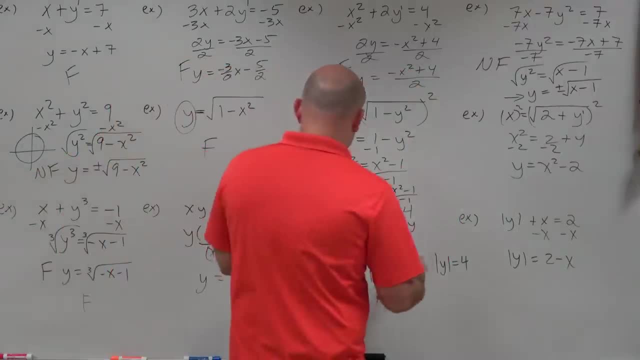 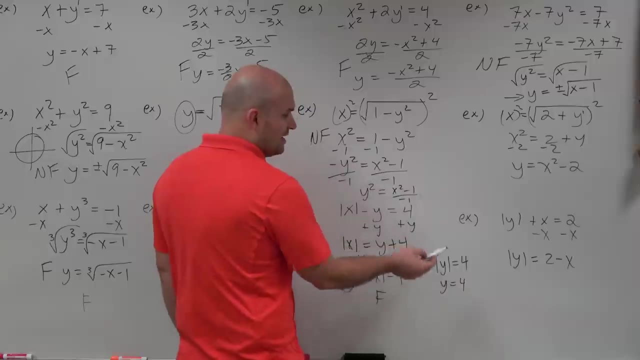 Now, what could be the values of y that equal 4?? Well, unlike the square roots, where you're inverse operation, we know that absolute value y could be y could equal 4.. Because if I plugged in 4 in for y, absolute value of 4 is 4.. 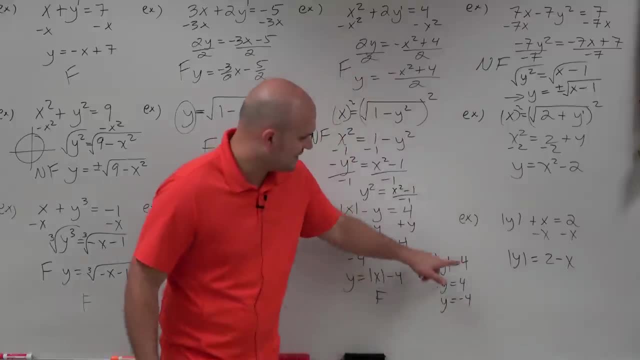 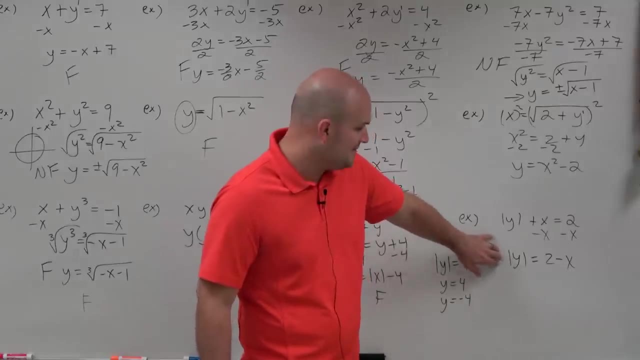 Also, though, y could equal negative 4. Because if I plug negative 4 in for y, absolute value of y is still equal to 4.. So what happens is, if I want to undo, I want to solve for y. 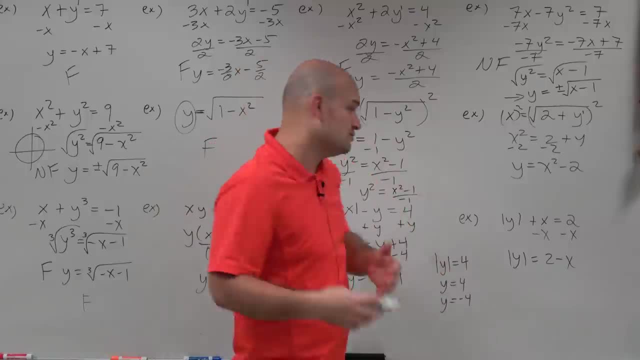 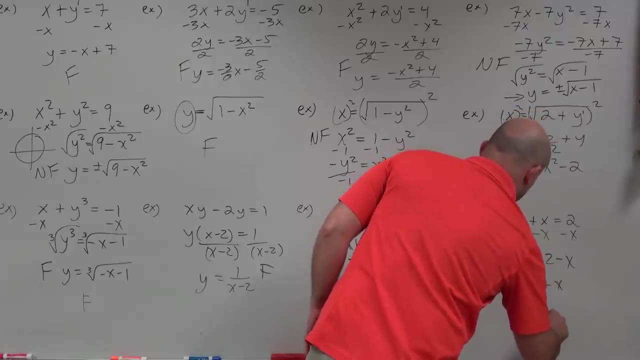 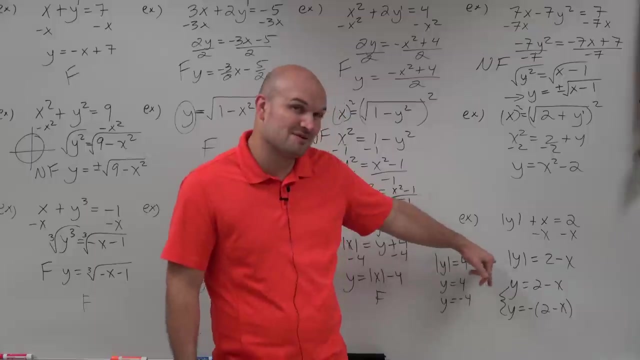 what I need to do to undo the absolute value. I basically need to create two solutions where y equals 2 minus x and y equals the opposite of 2 minus x. So what happens is by solving for y, by undoing the absolute value, I need to create 2 minus x. 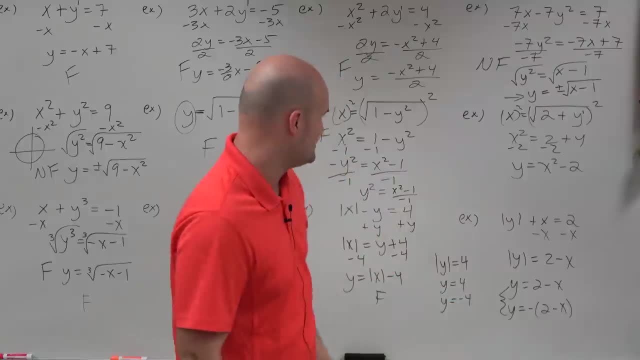 So what happens is by solving for y by undoing the absolute value, I need to create 2 minus x. So both Quer удeg like us, are that two different cases. so therefore y is not unique anymore, because now I have two cases, just like I. 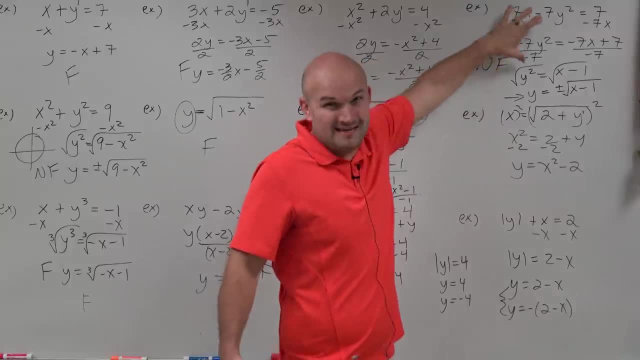 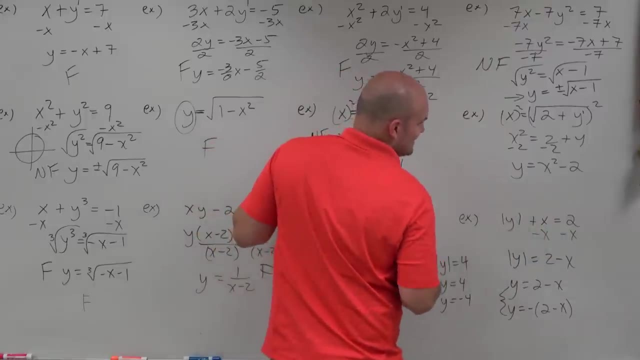 had two cases over here. So therefore, when you have y raised to an even power, it is not a function. When you have y inside an absolute value function, it is not a function. So for this video, that is the basic summary. 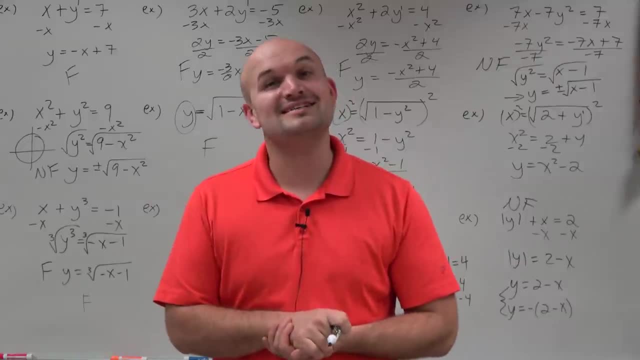 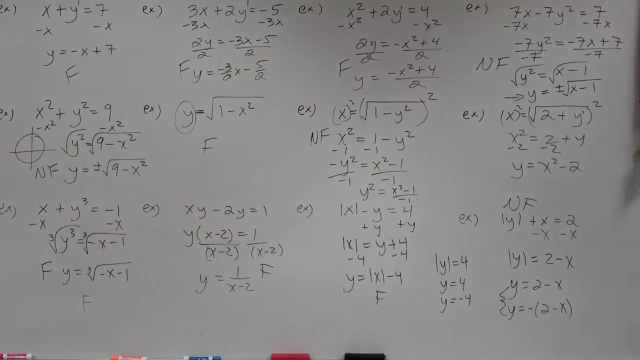 that I want you to take away. I hope you learned something and I hope you continue working hard, learning and staying curious. Thanks, Thank you. 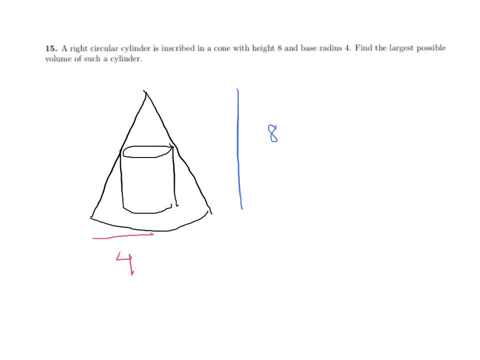 Okay, we have a right circular cylinder inside a cone, of height 8 and base radius 4. We have to figure out the largest possible volume of such a cylinder. We're going to go ahead and give some names to the dimensions of the cylinder. 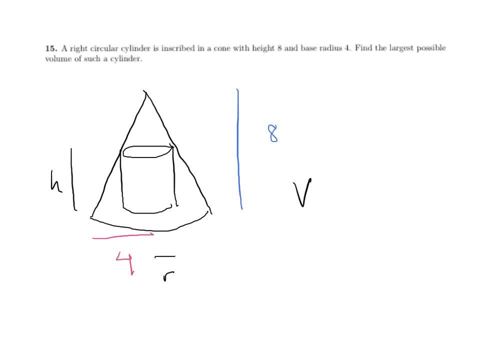 h for height, r for radius Volume is pi r squared h. That's our objective. Now the question is: what is the constraint? You can stare at this for a really long time before realizing what to do, So I'm just going to sort of give it away.